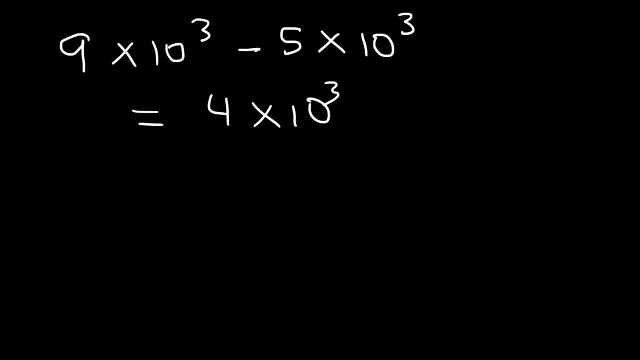 So this is simply going to be 4 times 10 to the 3.. You can do that if these two are the same. So go ahead and try these examples: What's 7 times 10 to the 4, plus 2 times 10 to the 3?? 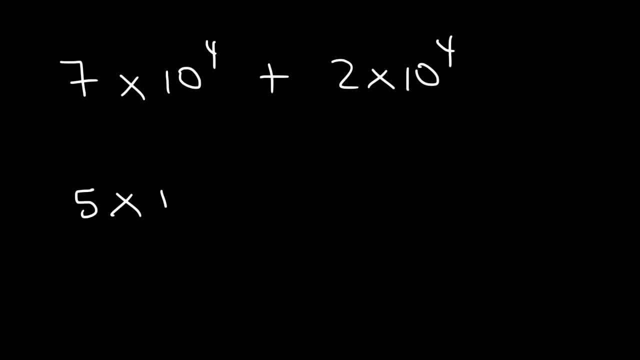 5 times 10 to the 4. And 5 times 10 to the 6, minus 3 times 10 to the 6.. So 7 plus 2 is 9.. And then the 10 to the 4 will be carried over. So that's the first answer. 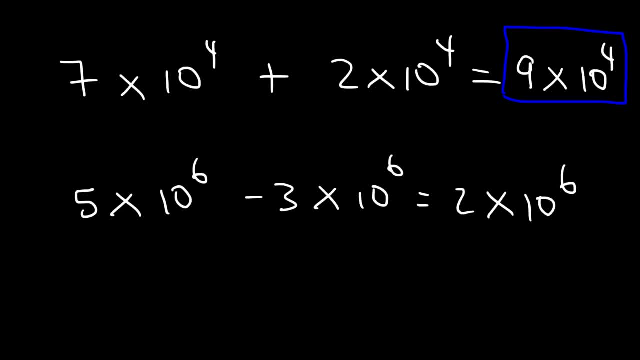 5 minus 3 is 2.. And so we're going to carry over the 10 to the 6.. And so that's a simple way to add or subtract two numbers in scientific notation. Now, what will we do Now? 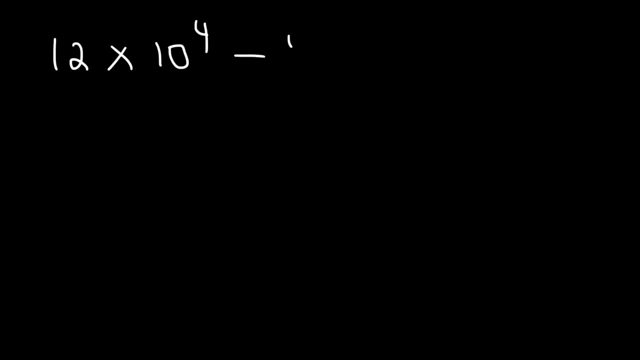 what will you do if the exponents are different? So what is 12 times 10 to the 4 minus 4 times 10 to the 5?? Right now, we cannot subtract 12 and 4, because these values are different. 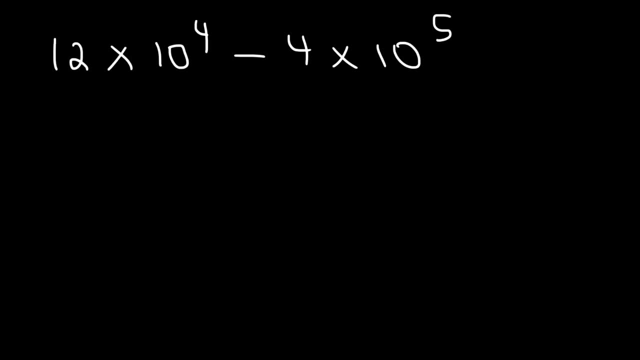 So what we need to do is to convert one into the other. So what I'm going to do is convert the smaller one into the larger one. So let's convert the 4. into a 5.. Now, if you move the decimal to the left, what's going to happen to the exponent? 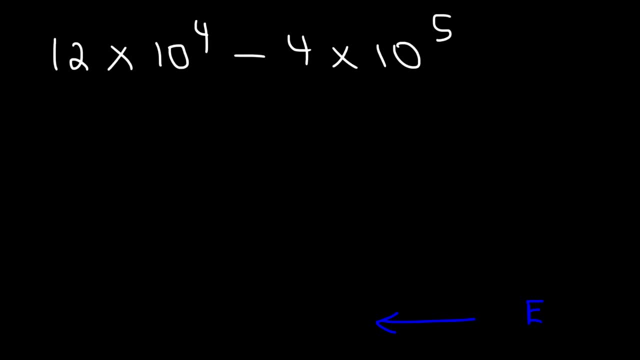 Will it increase in value or decrease in value? Any time you move the decimal to the left, the exponent will increase in value. As you move the decimal to the left, the number will decrease from 12 to 1.2, and so to undo. 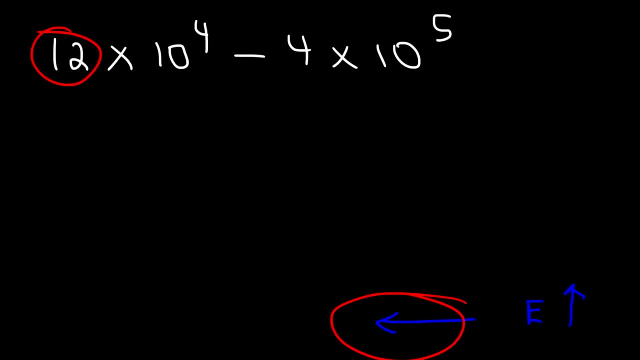 that to maintain balance, you need to increase the exponent. Likewise, if you increase the number by moving the decimal to the right, you need to decrease the exponent such that the value remains the same. So I'm going to move the decimal one unit to the left, and so 12 is going to decrease. 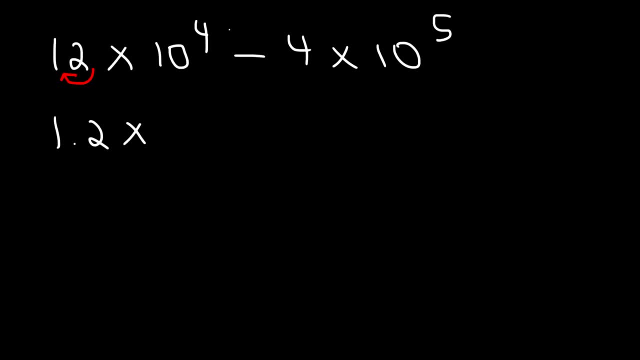 to 1.2, and so the exponent is going to increase by one. So now that these two are the same, I both have the 10 to the 5 multiplier. I can now subtract these two numbers. So what is 1.2 minus 4?? 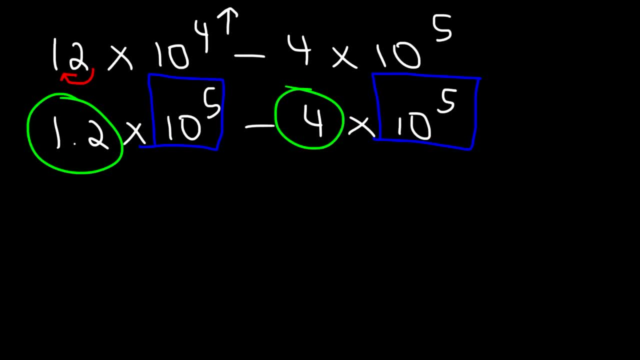 4 minus 1.2 is 2.8, so 1.2 minus 4 is going to be negative 2.8, and then this is going to be times 10 to the 5.. So that's the answer. 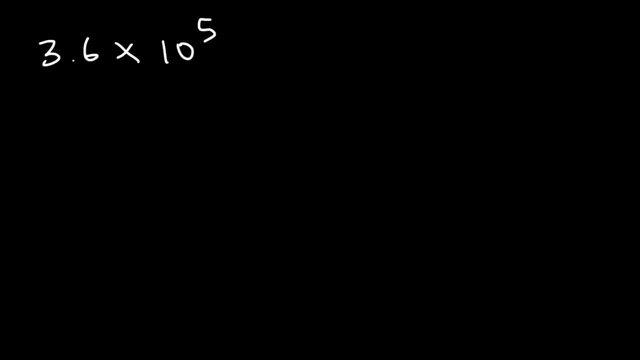 Let's try another example: 3.6 times 10 to the 5,, plus 10 to the 5.. So that's the answer, Plus 2.7 times 10 to the 4.. Go ahead and work on that example. 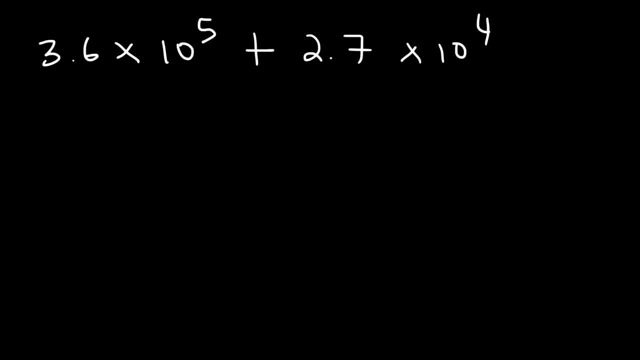 So I'm going to convert the smaller exponent into the larger one, So I'm going to move this decimal one unit to the left. so I'm going to decrease 2.7 to 0.27, so I need to increase the exponent to maintain the same value. 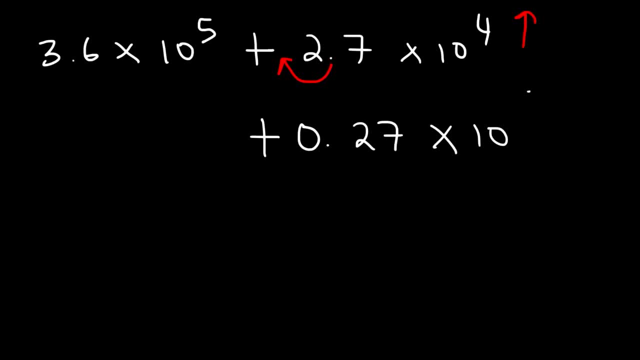 So this is going to be 0.27 times 10 to the 5.. So since I have the same multiplier, I can now add 3.6 with 0.27.. So this is going to be 7, 6 and 2 is 8,, 3 and 0 is 3.. 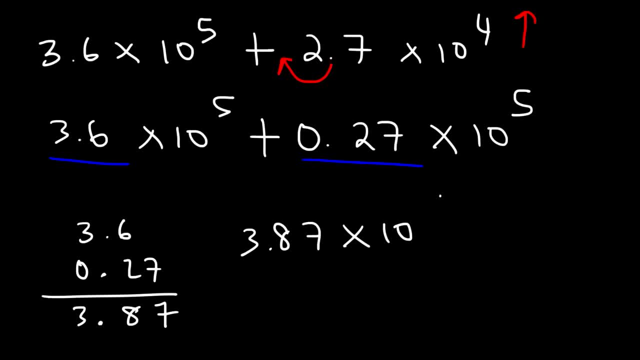 So this is going to be 3.87 times 10 to the 5.. And that's the solution. Subtitles by the Amaraorg community. Now, what about this one? 4.2 times 10 to the 7, plus 8 times 10 to the 5.. 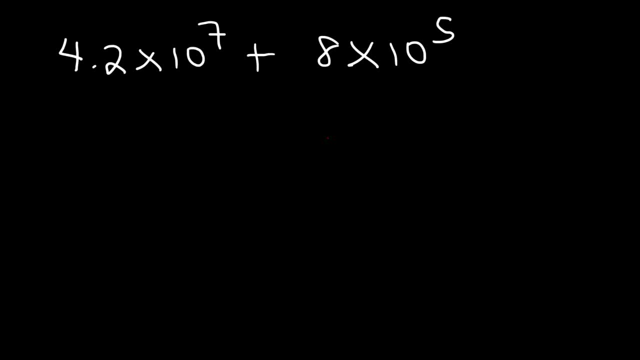 Go ahead and pause the video. So I'm going to move this decimal two units to the right: 1,, 2, so the exponent can increase by 2.. So I'm going to have a 0 here. This is going to become 0.08 times 10 to the 7.. 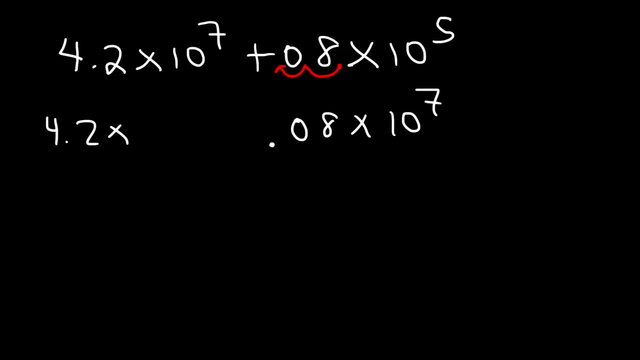 Subtitles by the Amaraorg community. Subtitles by the Amaraorg community. And so now I can add it with 4.2.. So 4.2 plus 0.08, that's going to be 4.28.. So it's 4.28 times 10 to the 7.. 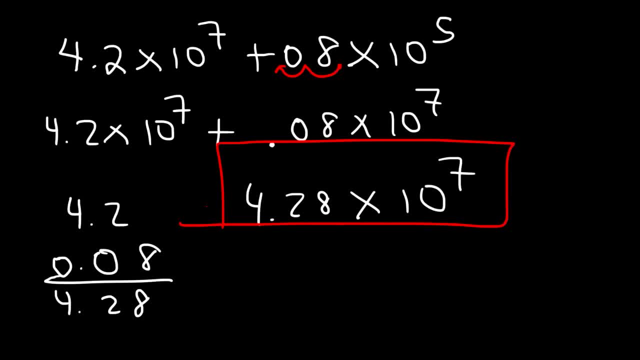 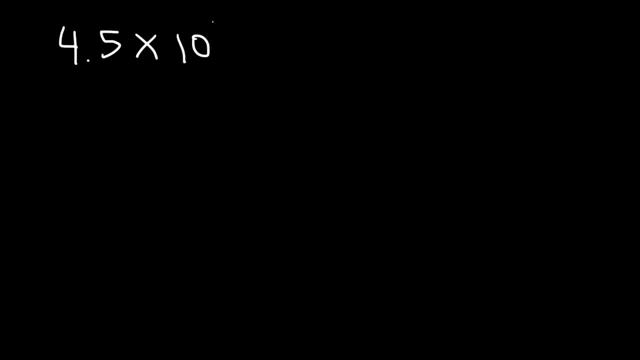 Subtitles by the Amaraorg community. And that concludes that problem. Let's try one more. So 4.5 times 10 to the 7 minus 8.2.. Subtitles by the Amaraorg community. Subtitles by the Amaraorg community. 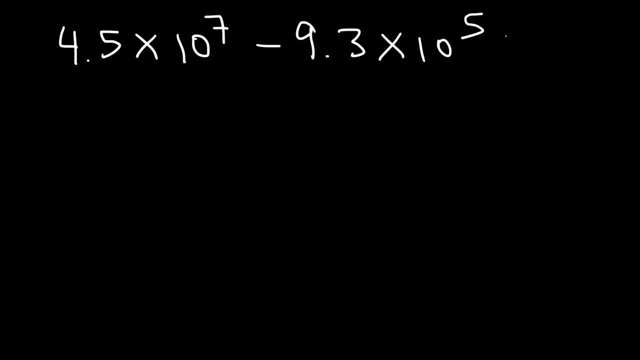 Minus 9.3 times 10 to the 5.. So I'm going to move this one 2 units to the left so I can get a 7.. This is going to increase by 2.. So there's going to be a 0 here. 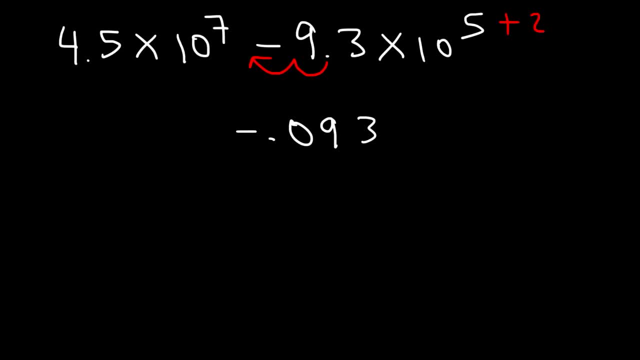 And so this is going to be 0.093 as opposed to 0.93 times 10 to the 7.. And so now let's subtract, And what's 4.5 minus 0.093? So we need to add some 0s. 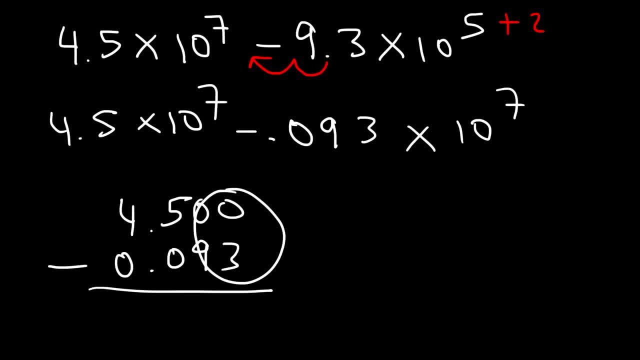 Now we can't subtract 0 by 3 because that's going to be negative, So we need to borrow a 1 to make this 10.. So we can't borrow a 1 from 0 because it's nothing, But we can borrow a 1 from 50.. 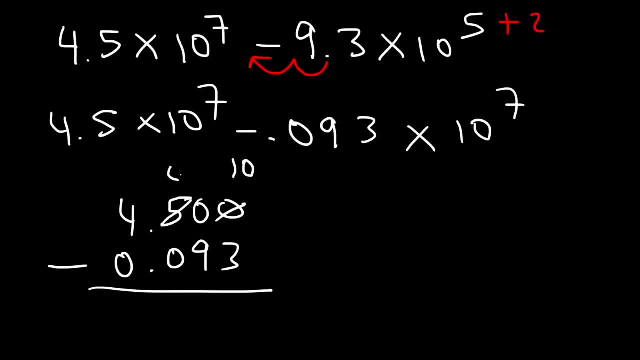 So that's going to become 49.. So this will be a 4 and this changes to a 9.. So now 10 minus 3 is 7.. 9 minus 9 is 0.. 4 minus 0 is 4.. 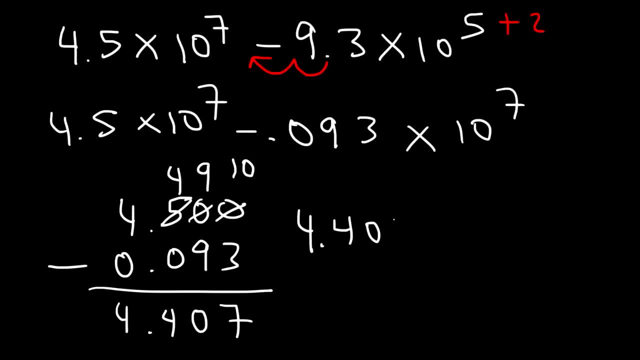 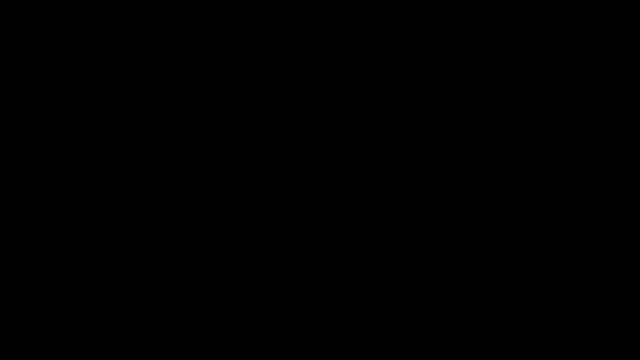 And this is also 4.. So it's going to be 4.407 times 10 to the 7.. So now you know how to add and subtract numbers using scientific notation. So you know they're going to be 0.. So now you know how to add and subtract the numbers. 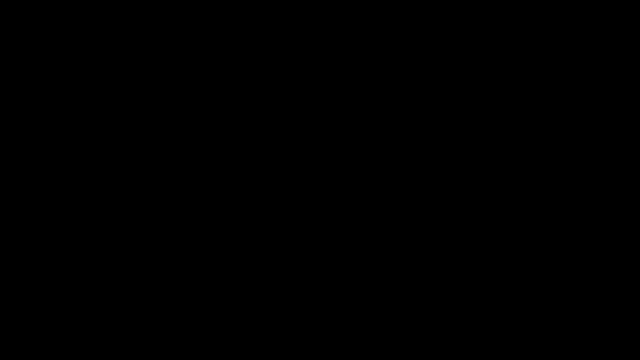 In the next lesson we'll explain how to make license codes. So all those things we learned today we'll use in theory on defined analysis. So if we can know which values are internal variables and what intensity values are internal variables, what intensity values are internal variables? this will be D-like, So we'll sayok racial vehicles uh. 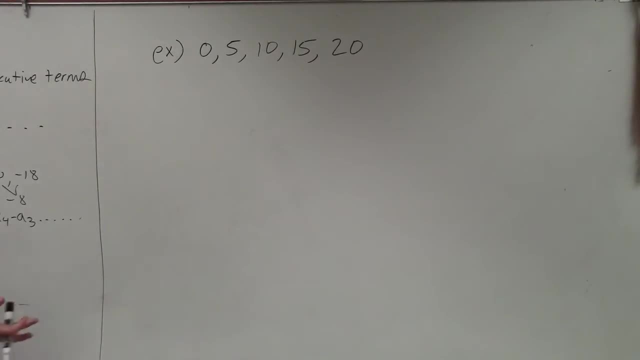 So in the next example, ladies and gentlemen, basically what we want to do is determine if this is an arithmetic sequence. So basically, ladies and gentlemen, all we're going to do this visually is we're just going to make sure that the difference between each of our terms is the